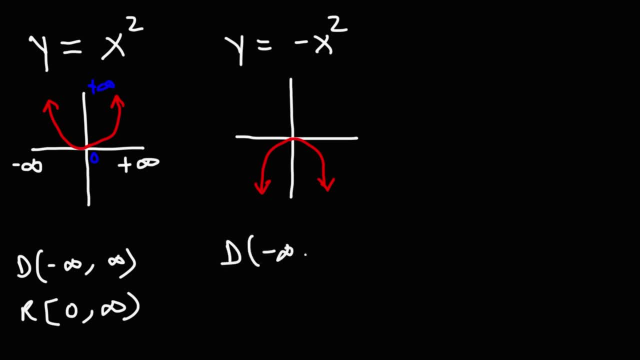 The domain is not going to change. It's going to be all real numbers. x could still take on any value, but the range is going to be different. The lowest y value is negative infinity. The highest y value is zero. So going from low to high is going to be from. 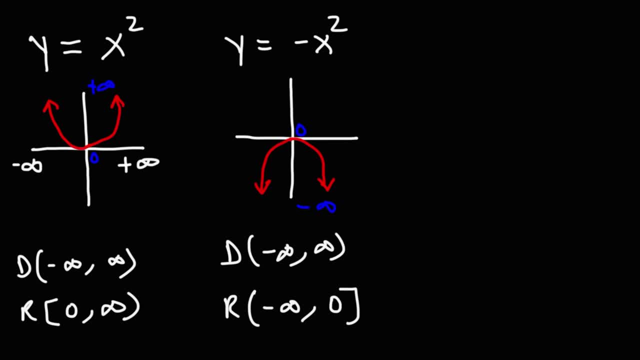 negative infinity to zero, but zero is included, so we're going to put a bracket at zero. So make sure you understand that. When finding the domain of a function, focus on the x values that the function can take on. When looking at the range of a function, focus on the y values that that function can take on. 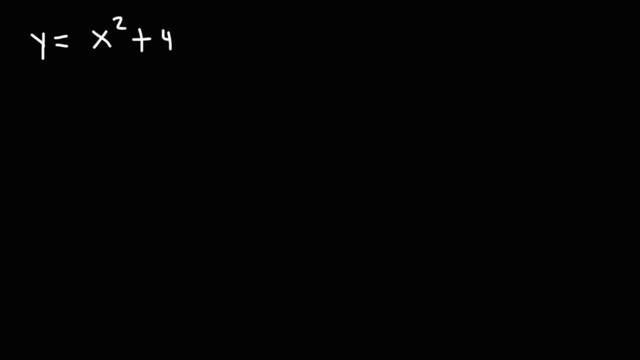 Now let's try another example. Let's say we have this function: y is equal to x squared plus four. Go ahead and find the domain and range for that function And then try this one. Feel free to pause the video if you want to try these. 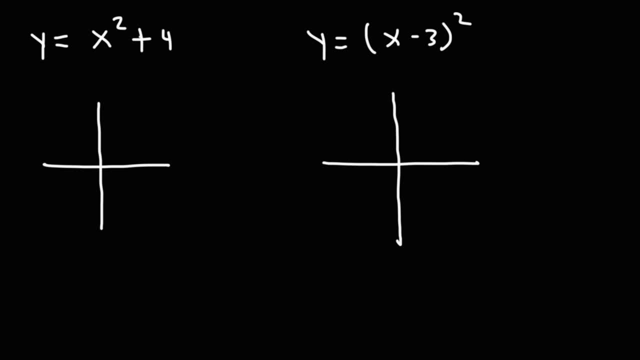 So now we're dealing with transformation of functions. So this one is basically x squared, but shifted four units up. So this is going to start at positive four And the graph is going to open upward. The domain is going to be the same thing. 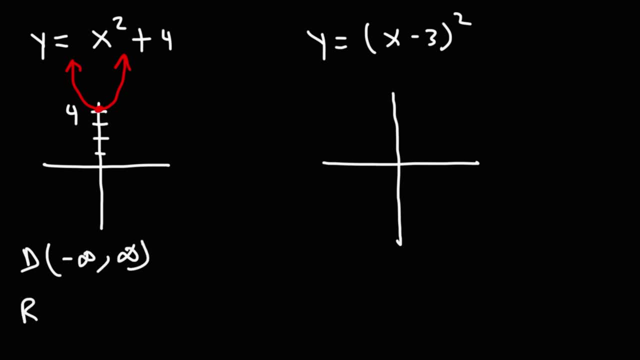 Negative infinity to infinity. The range is different. The lowest y value that we can see here is four, And the highest goes all the way up to infinity. So it's going to be four to infinity. Now for the next one. this is going to shift three units to the right. 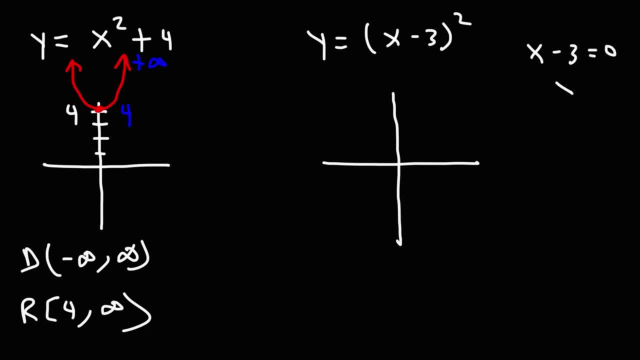 If you set the inside equal to zero, you'll get that x is equal to three. So the vertex will be at positive three on the x axis And because this is plus x squared, not minus x squared, the graph is going to open upward. 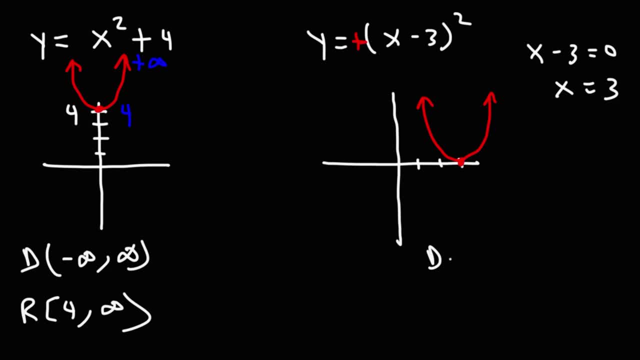 So the domain will still be the same- Negative infinity to infinity- But the range is going to be different. The lowest y value is zero, The highest is infinity. So it's going to go from zero to infinity. Go ahead and try these two examples. 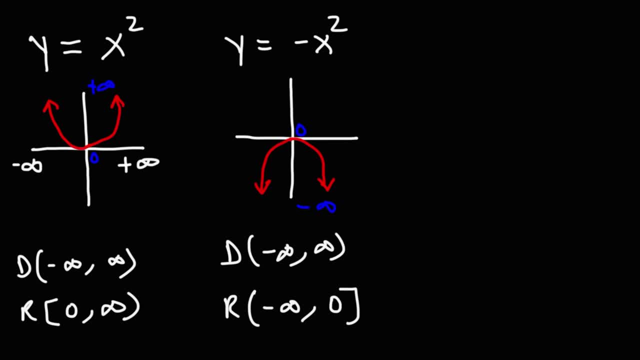 negative infinity to zero, but zero is included, so we're going to put a bracket at zero. So make sure you understand that. When finding the domain of a function, focus on the x values that the function can take on. When looking at the range of a function, focus on the y values that that function can take on. 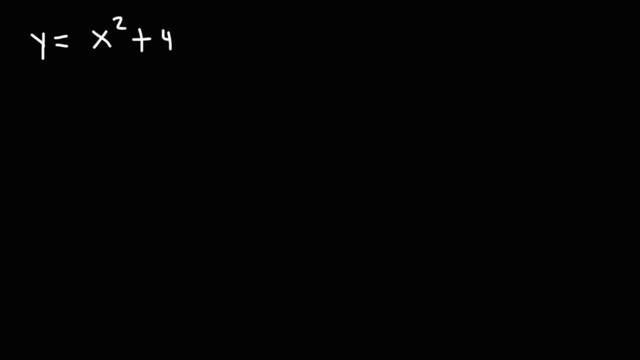 Now let's try another example. Let's say we have this function: y is equal to x squared plus four. Go ahead and find the domain and range for that function And then try this one. Feel free to pause the video if you want to try these. 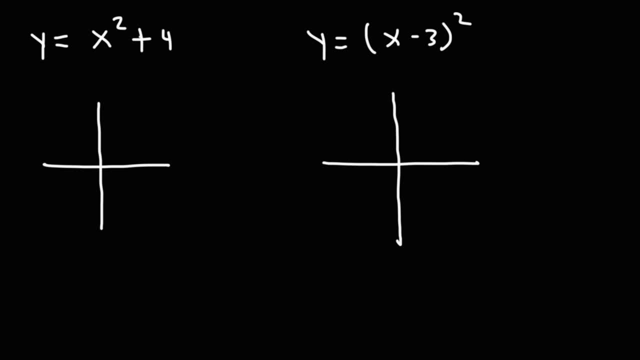 So now we're dealing with transformation of functions. So this one is basically x squared, but shifted four units up. So this is going to start at positive four And the graph is going to open upward. The domain is going to be the same thing. 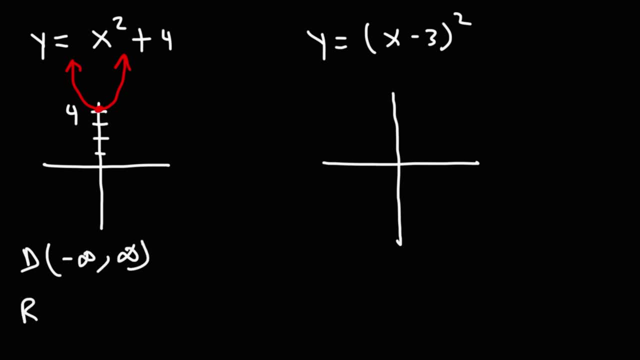 Negative infinity to infinity. The range is different. The lowest y value that we can see here is four, And the highest goes all the way up to infinity. So it's going to be four to infinity. Now for the next one. this is going to shift three units to the right. 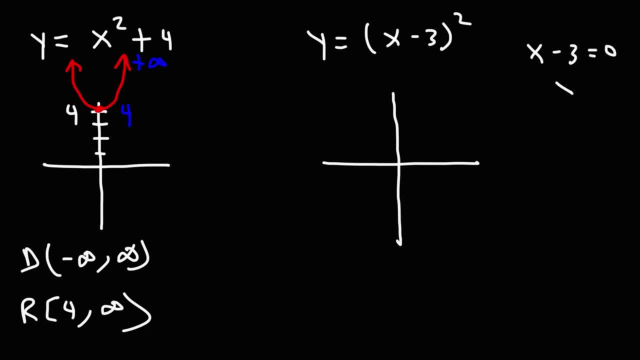 If you set the inside equal to zero, you'll get that x is equal to three. So the vertex will be at positive three on the x axis And because this is plus x squared, not minus x squared, the graph is going to open upward. 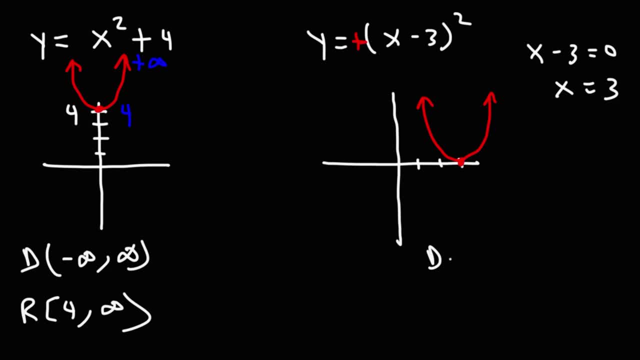 So the domain will still be the same- Negative infinity to infinity- But the range is going to be different. The lowest y value is zero, The highest is infinity. So it's going to go from zero to infinity. Go ahead and try these two examples. 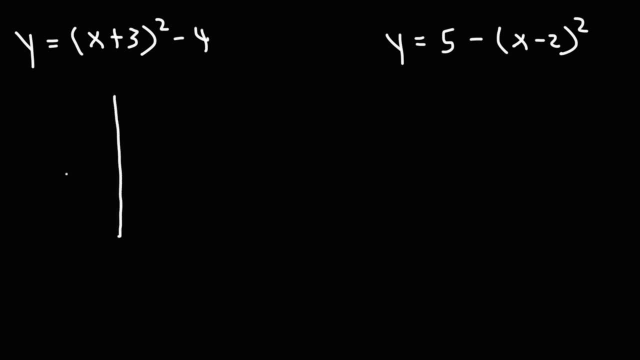 Now for the first one. on the left, we have x plus three instead of x minus three, So it's going to be shifted three units to the left. If you set x plus three equal to zero, you're going to get x is equal to negative three. 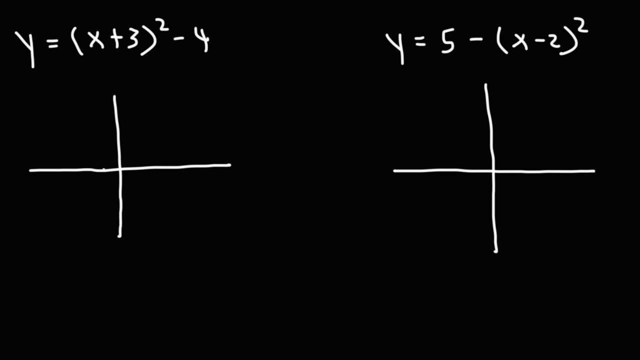 So we're going to shift three units to the left. So we're going to shift three units to the left. Now, this tells us that the graph is going to be shifted down four units. The point of interest that we need is the vertex. 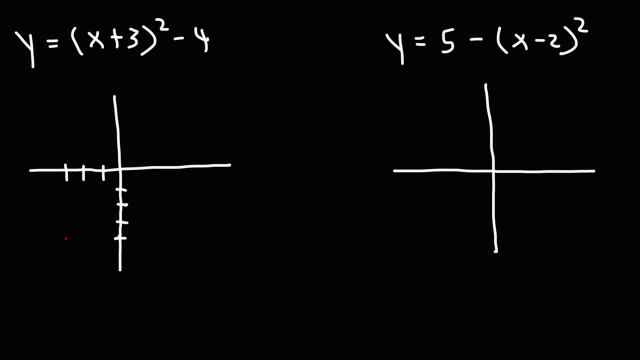 The vertex is going to be at an x value of negative three and a y value of negative four. Now we have a positive sign in front of the x squared term. If you were to FOIL it, you'll get positive x squared, And so this graph is going to open upward. 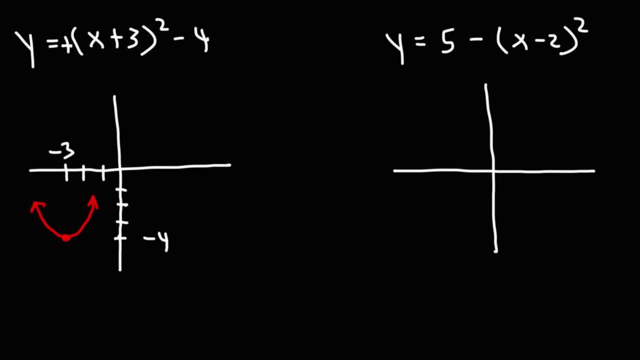 We don't need a perfect graph. We don't have to get all the points. All we need is the vertex and whether or not the graph is opening upward or downward. With that information we could find the domain and range of any quadratic function. 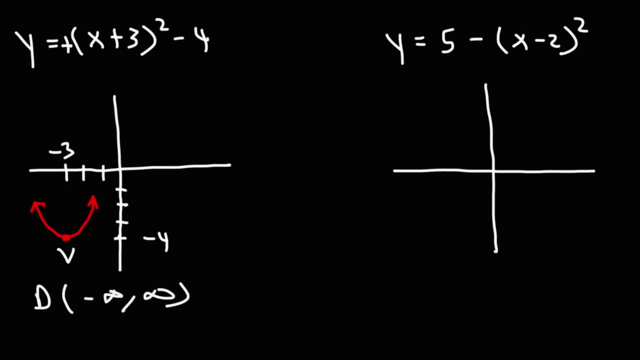 The domain is still going to be the same. Now for the range we could see. the lowest y value is negative four And this is going to keep going to positive infinity. So the range is from negative four to infinity. And so that's it for that example. 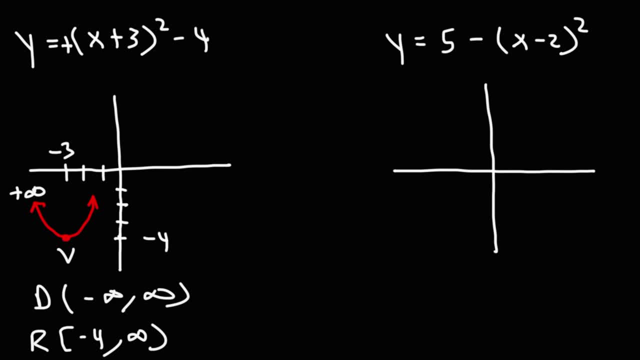 Now for the next one. we can see the graph is going to be shifted up five units. If you set x minus two equal to zero, you'll get x plus two. I mean x is equal to plus two. So it's going to be shifted to the right two units. 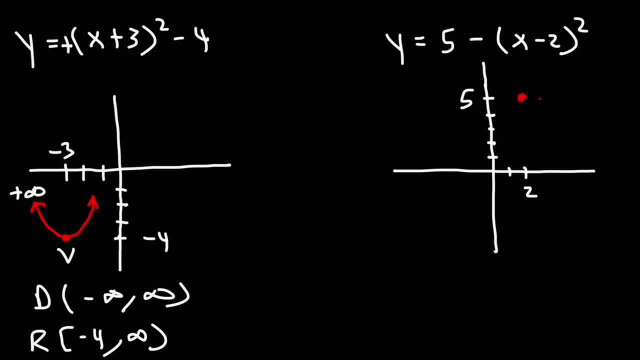 So the vertex will be at two comma five. Now we have a negative sign in front of the x squared term, So that tells us that this graph is going to open downward. So with this information we can now write the domain and range. 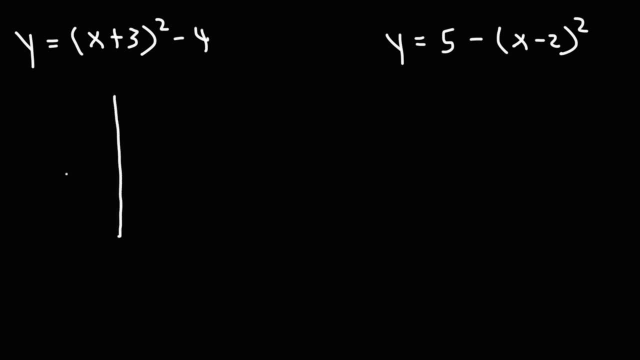 Now for the first one. on the left, we have x plus three instead of x minus three, So it's going to be shifted three units to the left. If you set x plus three equal to zero, you're going to get x is equal to negative three. 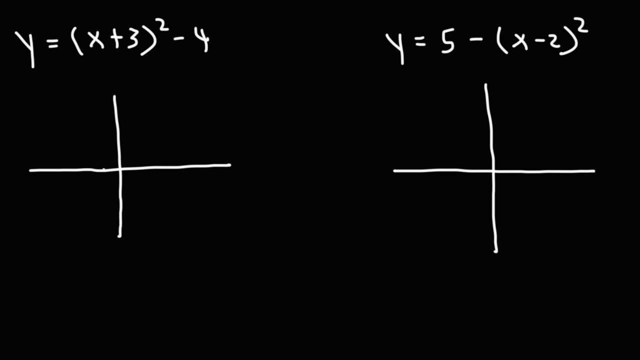 So we're going to shift three units to the left. So we're going to shift three units to the left. Now, this tells us that the graph is going to be shifted down four units. The point of interest that we need is the vertex. 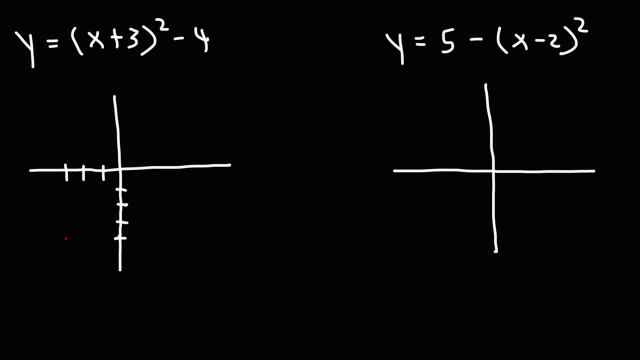 The vertex is going to be at an x value of negative three and a y value of negative four. Now we have a positive sign in front of the x squared term. If you were to FOIL it, you'll get positive x squared, And so this graph is going to open upward. 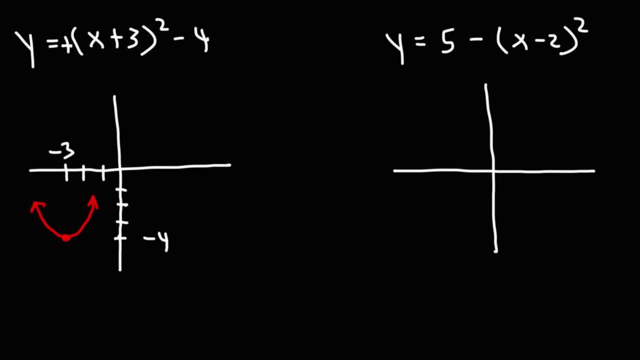 We don't need a perfect graph. We don't have to get all the points. All we need is the vertex and whether or not the graph is opening upward or downward. With that information we could find the domain and range of any quadratic function. 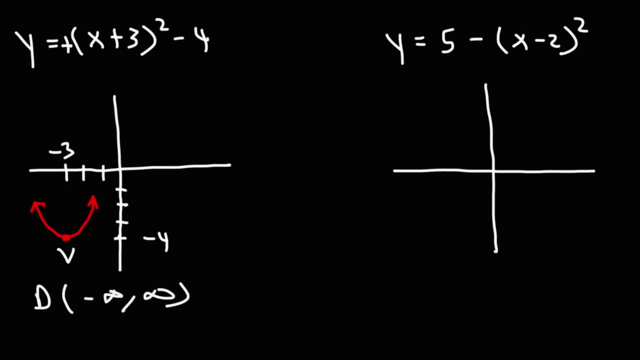 The domain is still going to be the same. Now for the range we could see. the lowest y value is negative four And this is going to keep going to positive infinity. So the range is from negative four to infinity. And so that's it for that example. 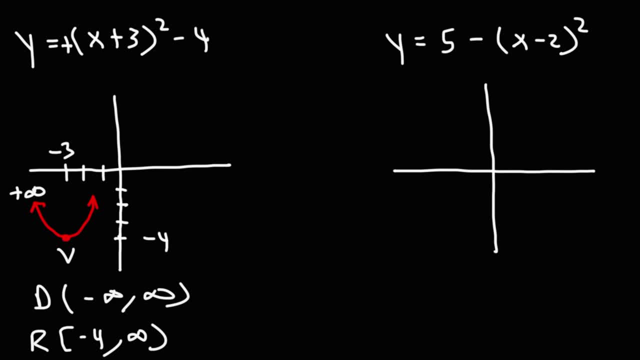 Now for the next one. we can see the graph is going to be shifted up five units. If you set x minus two equal to zero, you'll get x plus two. I mean x is equal to plus two. So it's going to be shifted to the right two units. 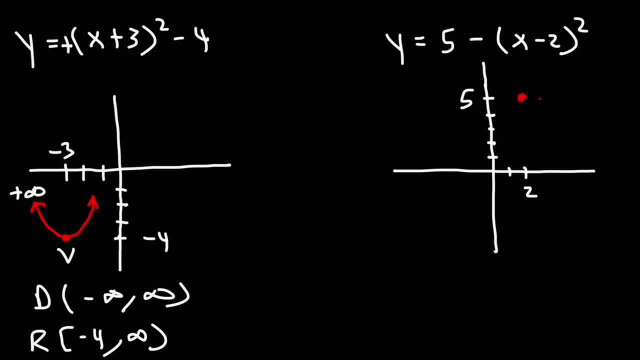 So the vertex will be at two comma five. Now we have a negative sign in front of the x squared term, So that tells us that this graph is going to open downward. So with this information we can now write the domain and range. 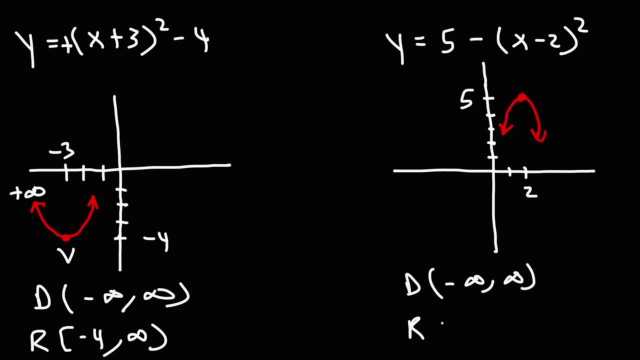 The domain is going to be all real numbers. The range: The highest Y value Is five, The lowest is going to be negative infinity. So looking at it from low to high, It's going to be negative infinity To five. 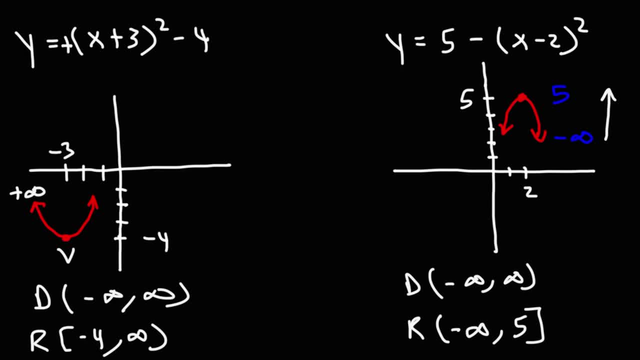 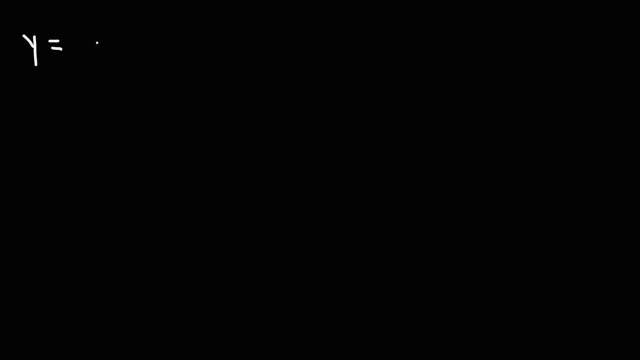 And five is included. So that's how you could find the range for that particular quadratic function. Now, sometimes you may receive a quadratic function In standard form As opposed to vertex form. So what would you do if you got a quadratic function that looked like that? 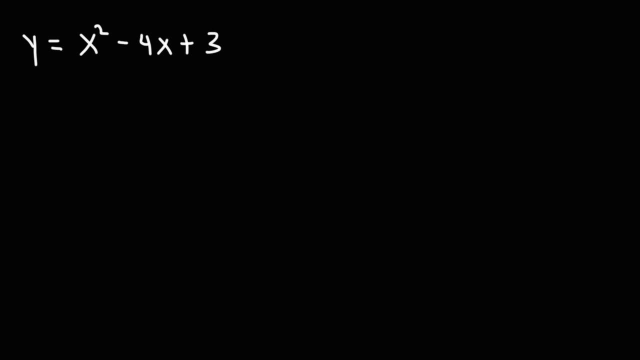 Well, you could factor it. This particular trinomial is factorable. Two numbers that multiply to the constant term three, But that add to the middle coefficient negative. four Are negative three and negative one. So to factor it, It's going to be x minus one. 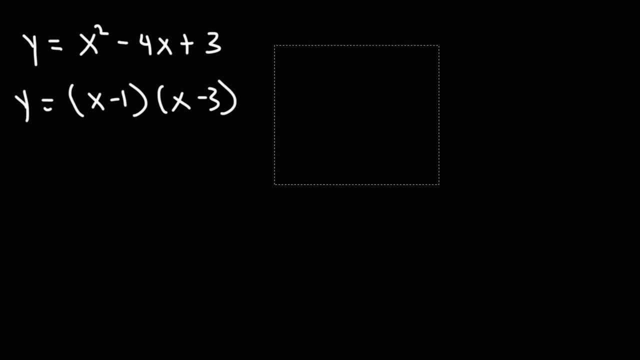 Times x minus three. If you set y equal to zero, You can get the x intercepts, Which will be at one And at three. The vertex will be at the midpoint Of The x intercepts, So the vertex Will have the x coordinate. 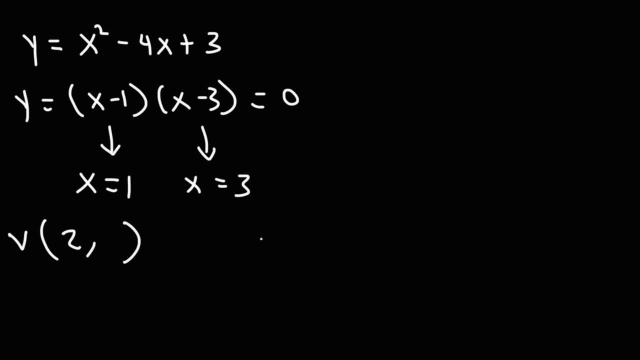 X equals two. Now we need the y coordinate of the vertex. So using the original equation, If we plug in two We can get the y coordinate. Now this point is very important For getting the range, Because the range is dependent. 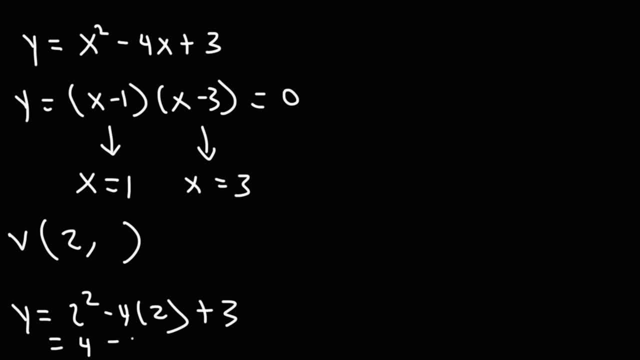 On the y value of the vertex. Four minus eight is negative, four Negative. four plus three Is negative one. So the vertex is two negative one And this is positive, x squared. So the graph is going to open upward. So now we can draw. 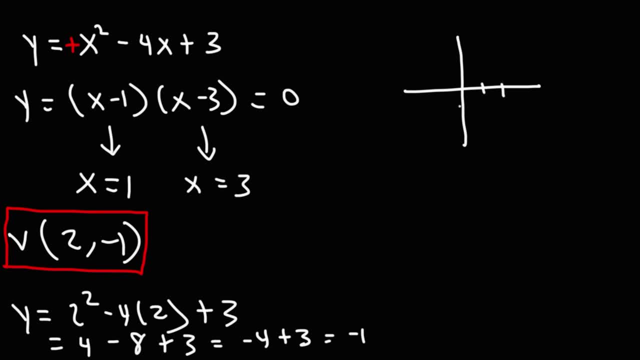 A rough sketch. I would plot the vertex Which is here, Two negative one, And we know it's going to open upward. Now we also know the intercepts, So we can plot that as well. We have an intercept at x equal one. 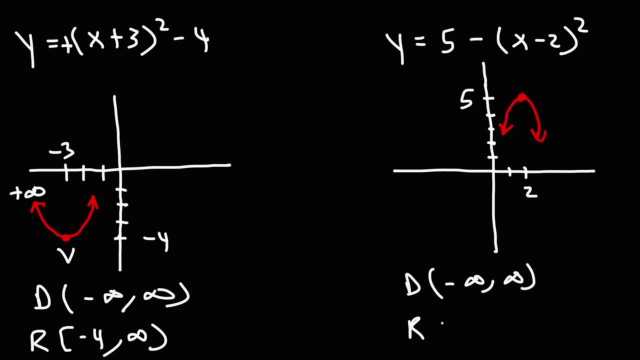 The domain is going to be all real numbers. The range: The highest Y value Is five, The lowest is going to be negative infinity. So looking at it from low to high, It's going to be negative infinity To five. 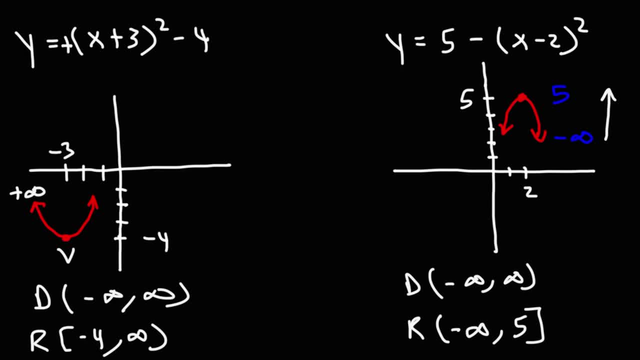 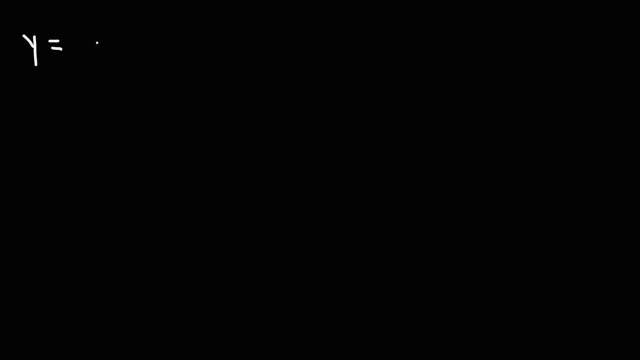 And five is included. So that's how you could find the range for that particular quadratic function. Now, sometimes you may receive a quadratic function In standard form As opposed to vertex form. So what would you do if you got a quadratic function that looked like that? 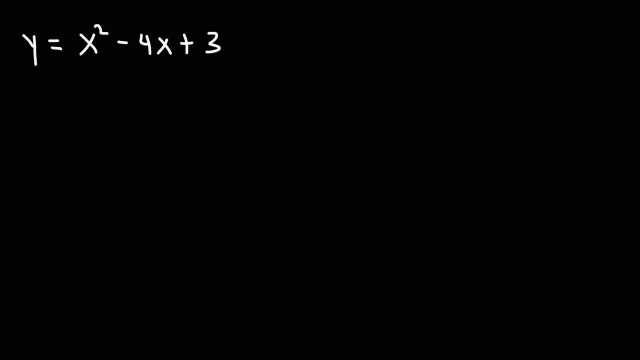 Well, you could factor it. This particular trinomial is factorable. Two numbers that multiply to the constant term three, But that add to the middle coefficient negative. four Are negative three and negative one. So to factor it, It's going to be x minus one. 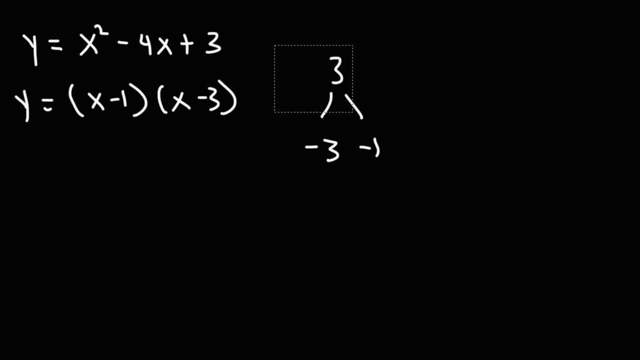 Times x minus three. If you set y equal to zero, You can get the x intercepts, Which will be at one And at three. The vertex will be at the midpoint Of The x intercepts, So the vertex Will have the x coordinate. 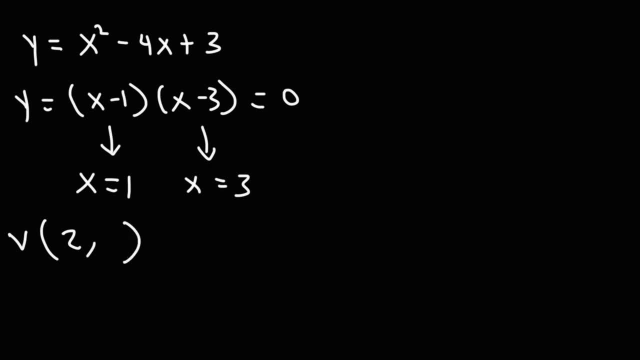 X equals two. Now we need the y coordinate of the vertex. So using the original equation, If we plug in two We can get the y coordinate. Now this point is very important For getting the range, Because the range is dependent. 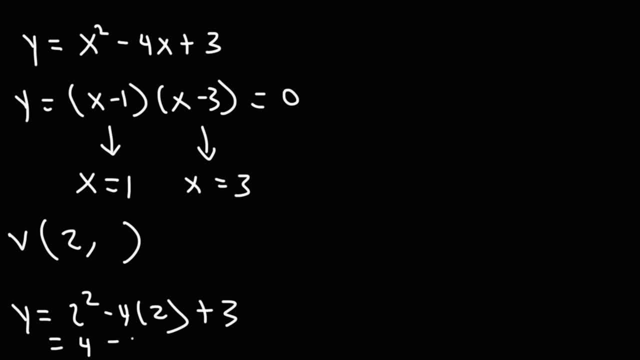 On the y value of the vertex. Four minus eight is negative, four Negative. four plus three Is negative one. So the vertex is two negative one And this is positive, x squared. So the graph is going to open upward. So now we can draw. 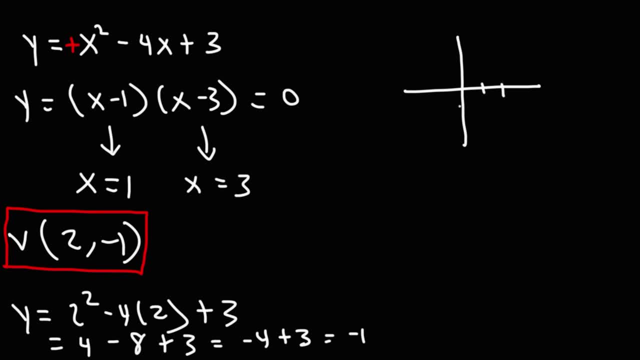 A rough sketch. I would plot the vertex Which is here, two negative one, And we know it's going to open upward. Now we also know the intercepts, So we can plot that as well. We have an intercept at x equal one. 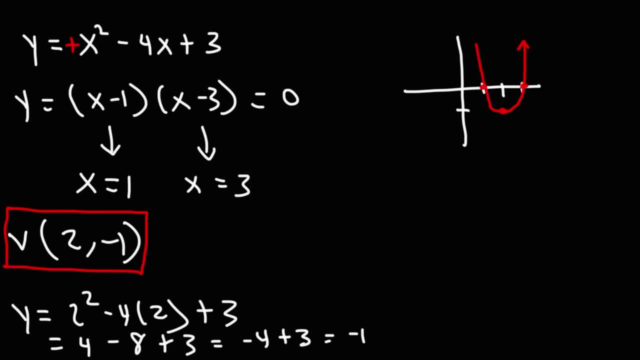 And x equal three And the graph is going to open In this general direction. So the domain, as always, Will be negative: infinity To infinity for a quadratic function. Now for the range We can see. the lowest y value Is negative one. 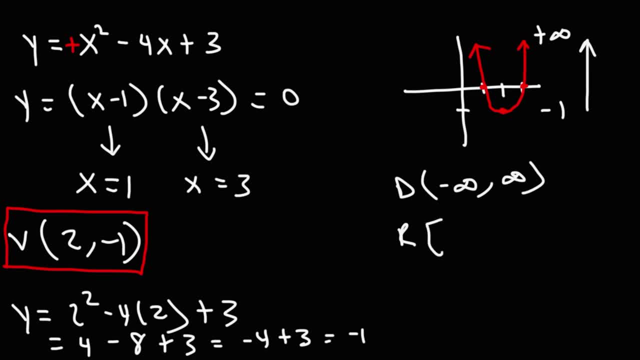 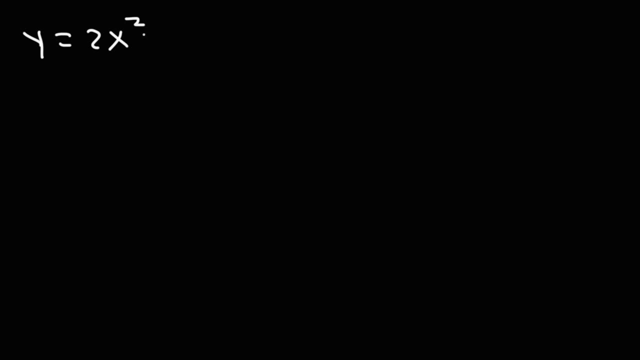 The highest is infinity. So we're going to go from Negative one to infinity. So that's it for this example problem. Now let's try one more. Let's say we have another Quadratic function that is In standard form. 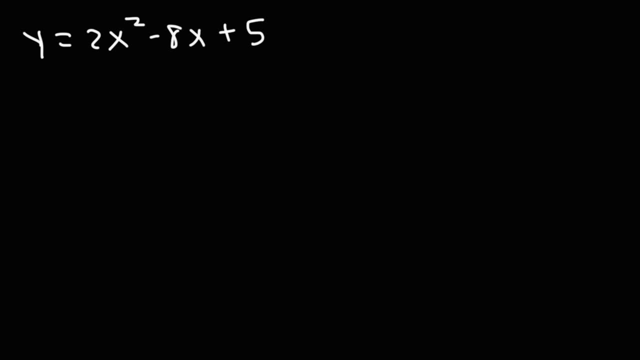 But it's not factorable. In this case You want to use this formula To get The x coordinate of the vertex. X is equal to negative b over two a, So a is two, B is negative eight, C is five. 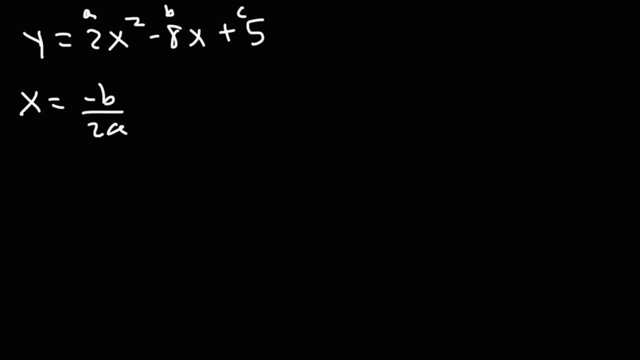 So this works If you're given the quadratic function In standard form Or in ax squared plus bx plus c format. So let's replace b with negative eight And a with two, So this becomes eight over four, Which is two. 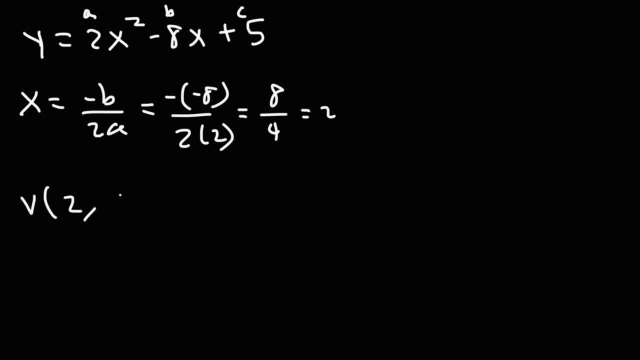 So the x coordinate of the vertex Is two. So now we got to find the y coordinate Of the vertex. So let's plug in two into that equation. Two squared is four times two is eight. Eight times two is sixteen. Eight minus sixteen is negative eight. 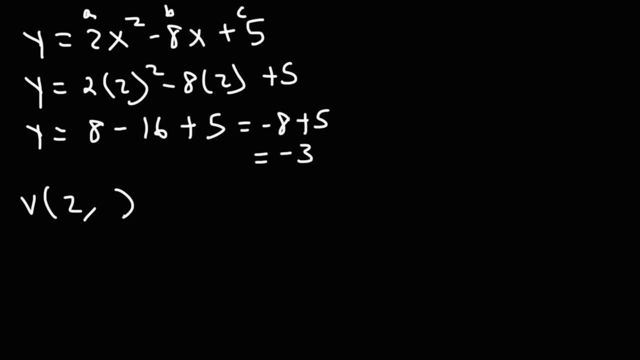 And negative eight plus five Is negative three. So we have a vertex Which is at two negative three And this is positive x squared, So it's going to open upward. So here's the vertex, And the graph is going to go in the upward direction. 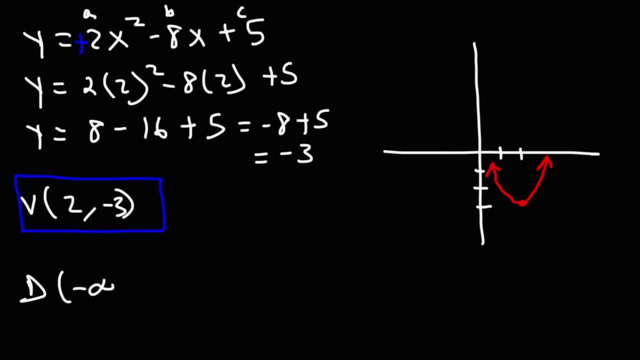 So the domain is going to be Our real numbers And the range We can see. the lowest y value is negative three And it's going to keep going All the way to positive infinity. So It's going to go from negative three to infinity. 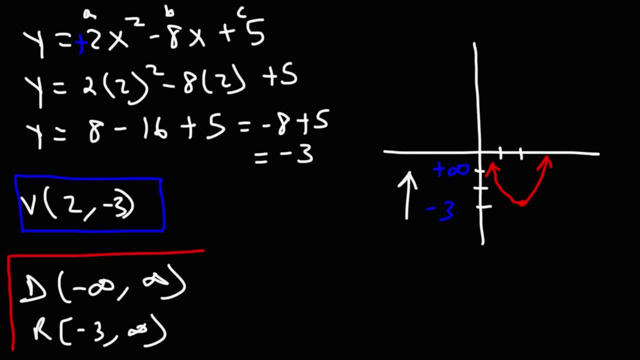 So that's basically it for this video. Now you know how to find the domain and range For any quadratic function. 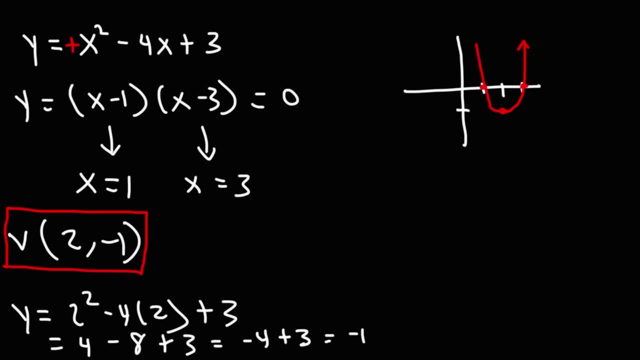 And x equal three And the graph is going to open In this general direction. So the domain, as always, Will be negative: infinity To infinity. for a quadratic function, Now for the range: The lowest y value is negative one, The highest is infinity. 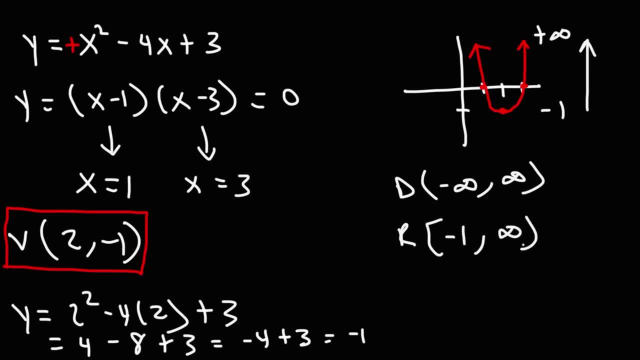 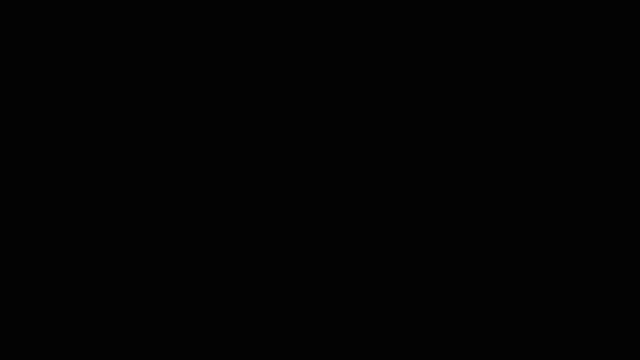 So we're going to go from Negative one to infinity. So that's it for this example problem. Now let's try one more. Let's say we have another Quadratic function that is In standard form But it's not factorable. 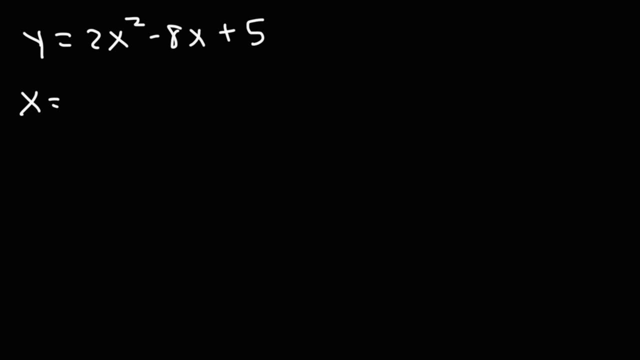 In this case You want to use this formula To get The x coordinate of the vertex. X is equal to negative b over two a, So a is two, B is negative eight, C is five. So this works If you're given the quadratic function. 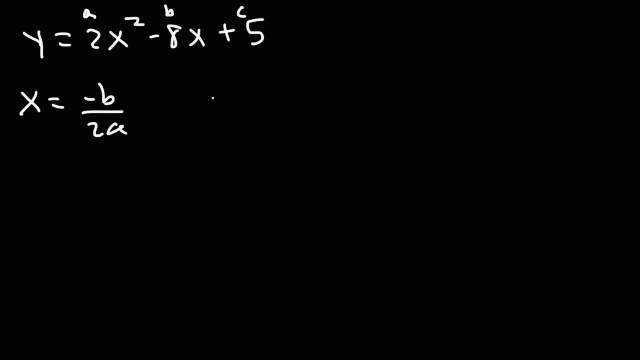 In standard form Or in ax squared plus bx plus c format. So let's replace b with negative eight And a with two, So this becomes Eight over four, Which is two. So the x coordinate of the vertex Is two. 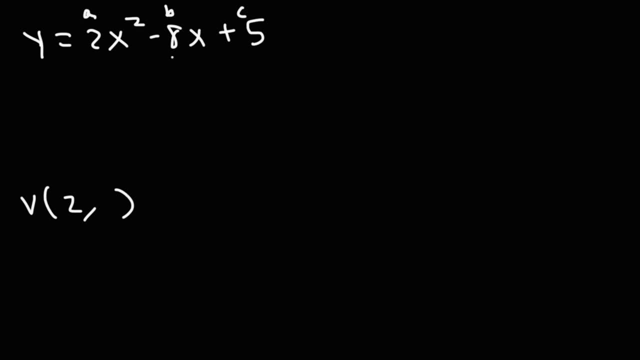 So now we've got to find The y coordinate of the vertex. So let's plug in two into that equation. Two squared is four times two is eight. Eight times two is sixteen. Eight minus sixteen is negative eight And negative eight plus five. 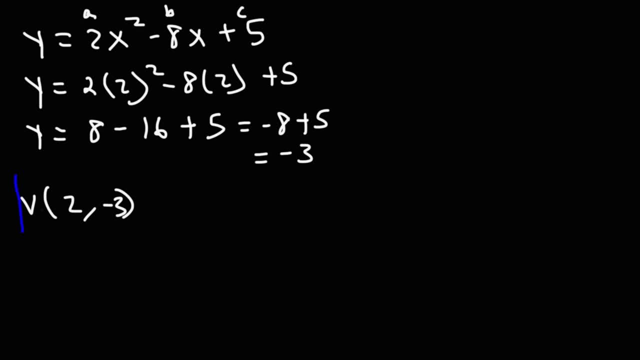 Is negative three. So we have a vertex Which is at two negative three And this is positive x squared, So it's going to open upward. So here's the vertex And the graph is going to go In the upward direction. 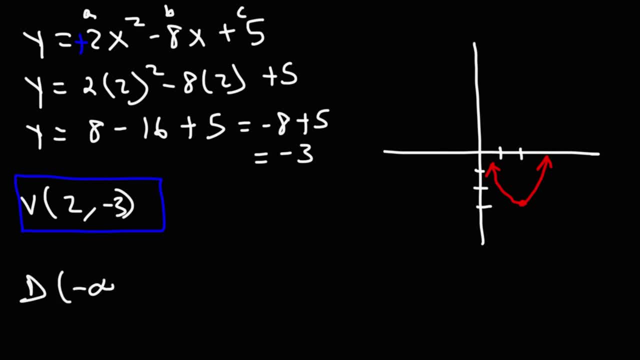 So the domain Is going to be all real numbers And then The range You can see, the lowest y value Is negative three And it's going to keep going All the way to positive infinity. So It's going to go from negative three 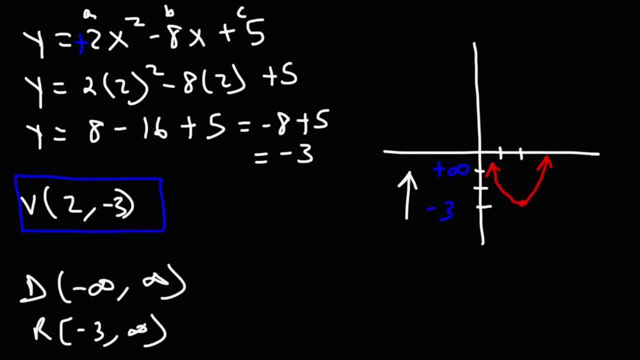 To infinity. So that's basically it for this video. Now you know how to find the domain and range For any quadratic function.